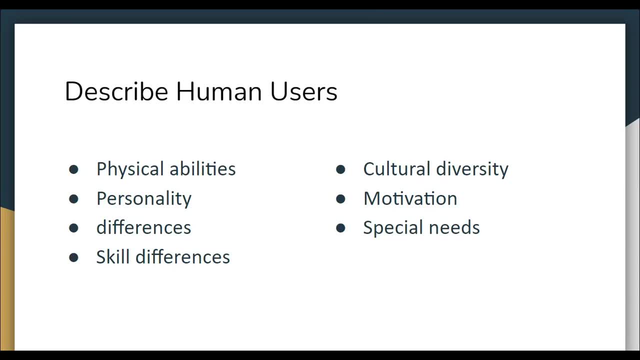 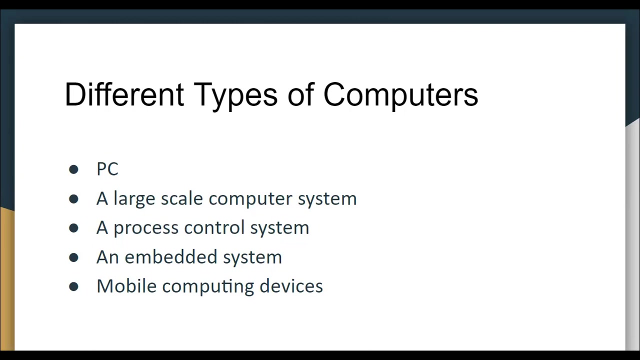 And also we can describe human users as follows: physical abilities, personality differences, skill differences, cultural diversity, motivation, special needs. Then let's see what are the different types of computer. Actually, there are a lot of types of computers in the market. 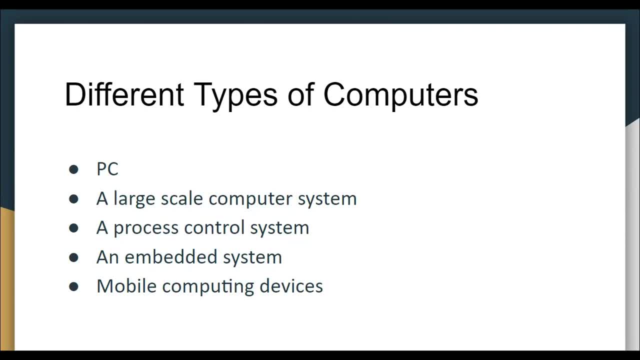 Let's see what are those. Firstly, PC, For example laptops, desktop PDA and a large-scale computer system, a process control system, an embedded system. mobile computing devices, For example wearable computers, mobile phone devices are some of these. 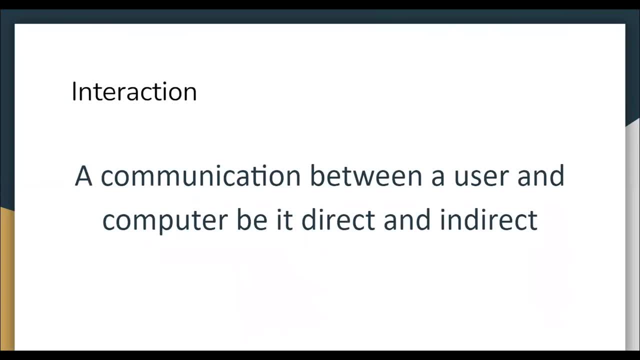 Then next we will see. what does the interaction mean. Interaction means a communication between a user and the computer. Actually, we will describe that in the previous video also. Then interaction we can divide as direct and indirect. Direct means a dialogue with feedback. 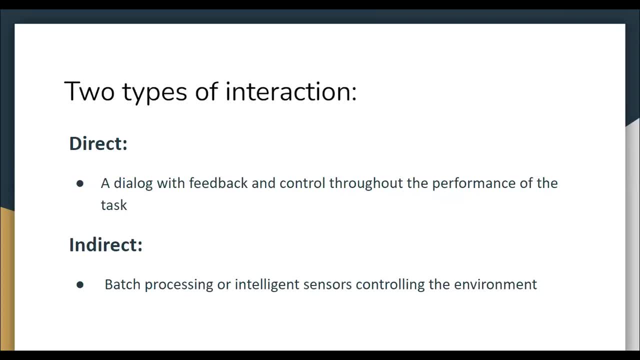 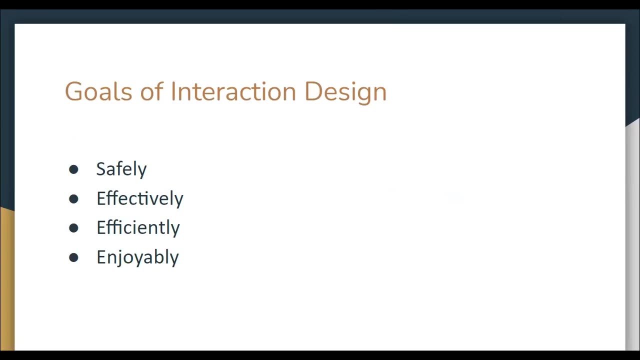 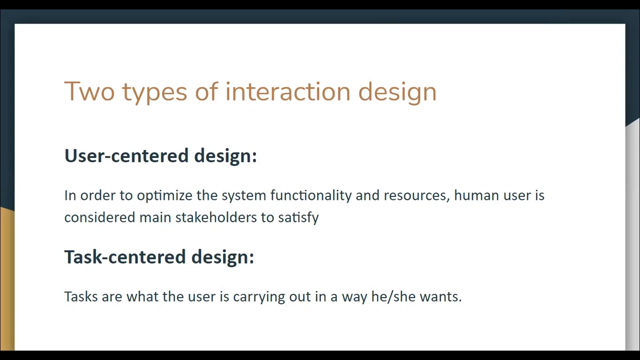 and control throughout the performance of the task. Indirect means batch processing or intelligent sensors controlling the environment. Then we will see what are the goals of interaction design: Safely, effectively, efficiently and enjoyably. Next, there are two types of interaction design. 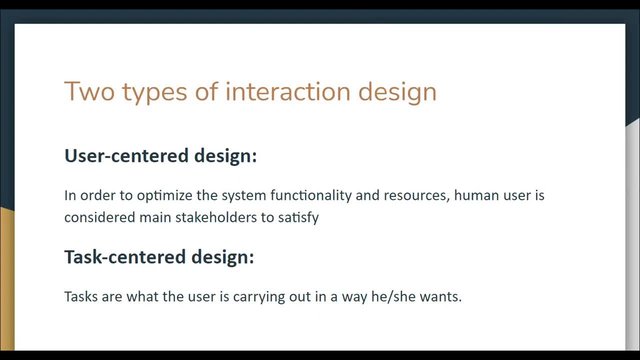 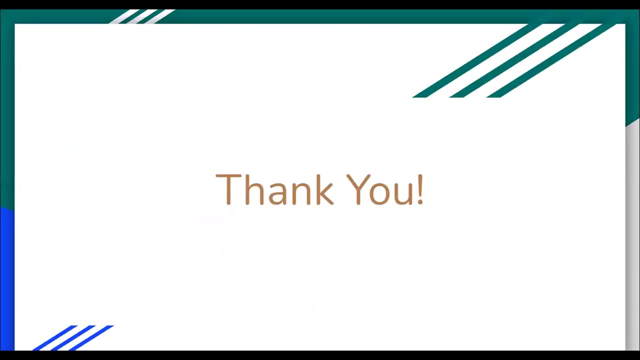 user-centered design. task-centered design. User-centered design means: in order to optimize the system functionality and resources, human user is considered main stakeholders to satisfy. Task-centered design means tasks are what the user is carrying out in a way he or she wants.